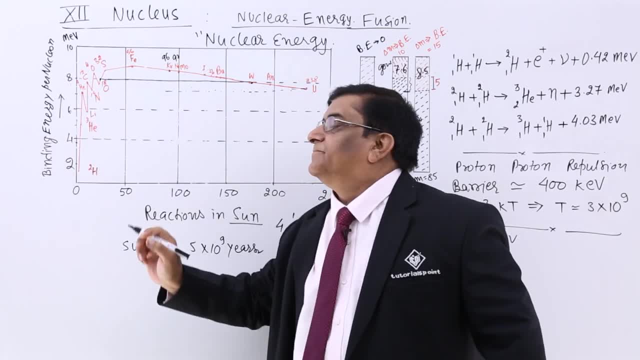 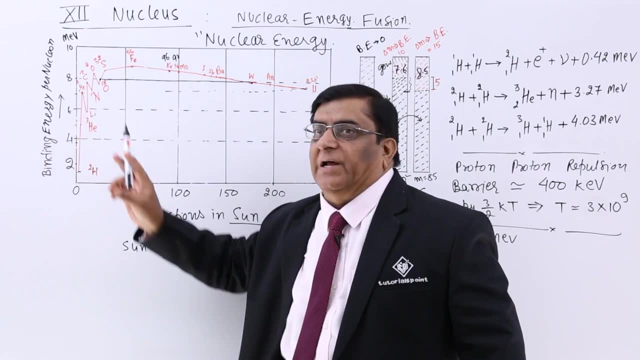 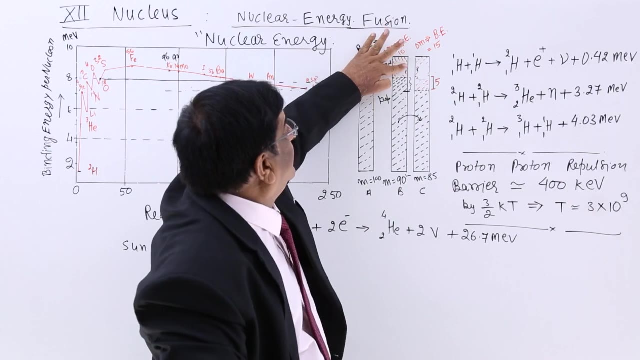 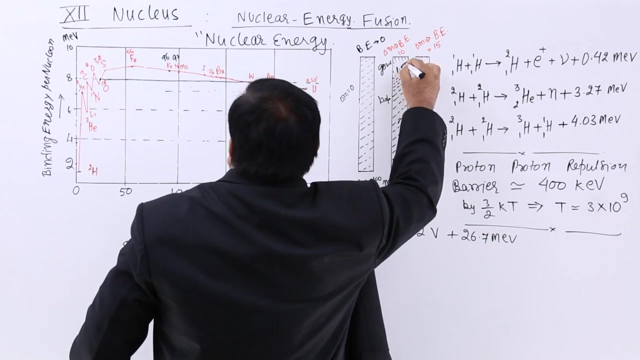 2 makes 4,, 4 helium. The binding energy for hydrogen is very small, the binding energy for helium is very large and when the binding energy is small to binding energy large, if we go, then we get the energy. And this was here, say 1.5, and this is here, say it is 7.2. so for every 1 fusion for 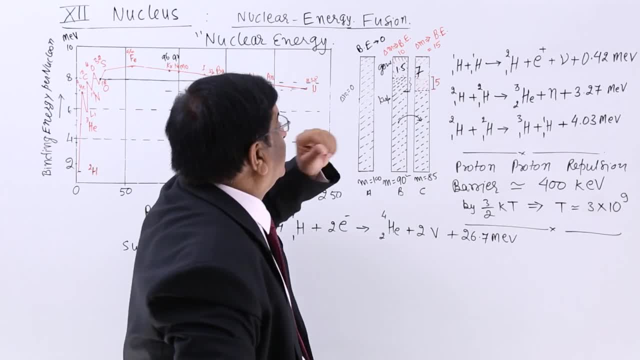 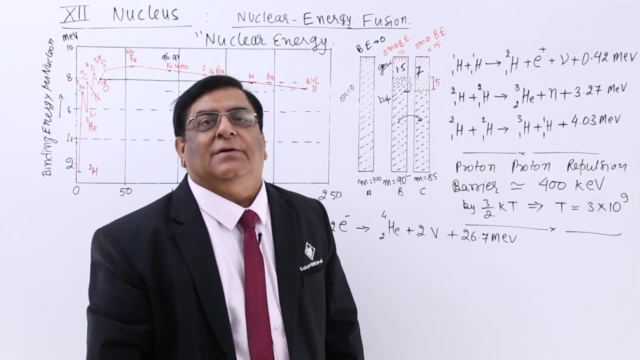 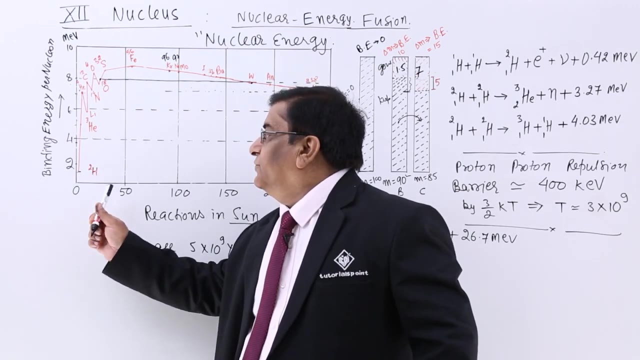 every 1 fusion we get a very large amount of energy, say around 4.5.. So what happens in it? This hydrogen, nuclear, which is the 1.5 hydrogen. it becomes a small concentration of hydrogen and this get air is a proton, and here we have two, so there is one proton and one neutron, these two and 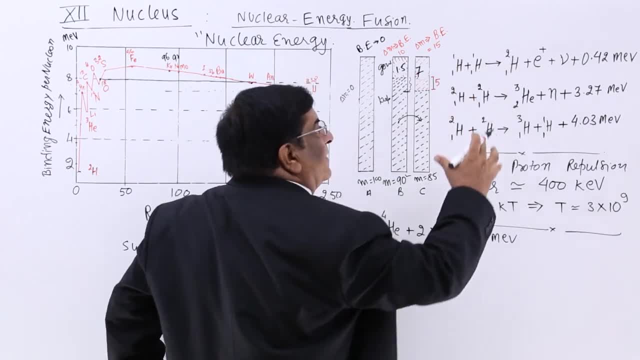 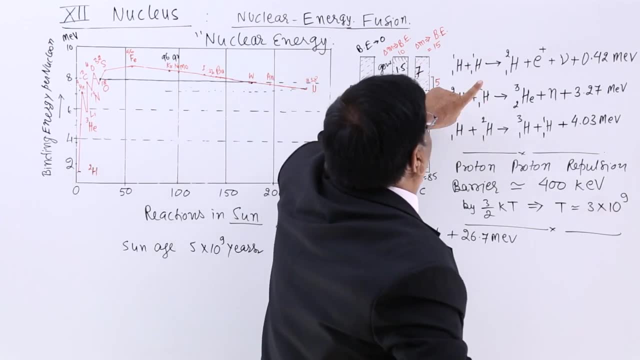 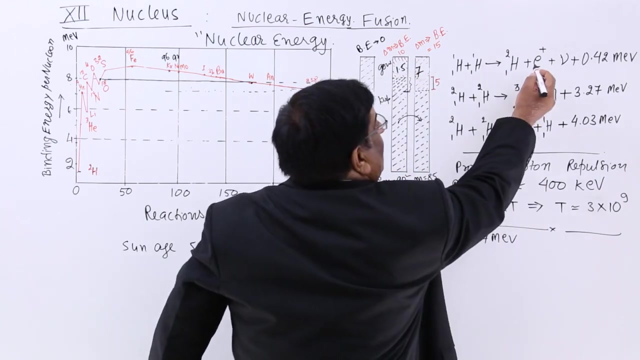 they are brought together. here it is. there are so many reactions taking place in it and we have written it step by step. first one hydrogen, one proton, only one proton only. they combine together and make hydrogen. with mass 2, one electron is released. sorry, one positron. 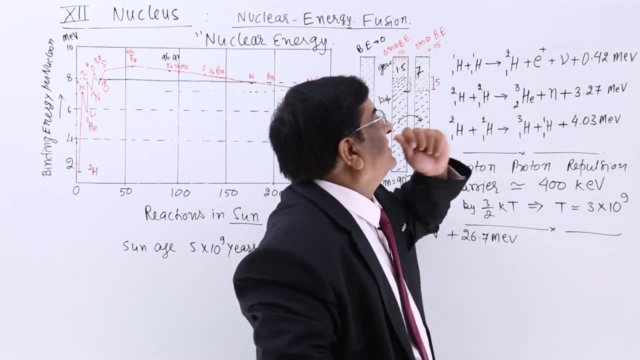 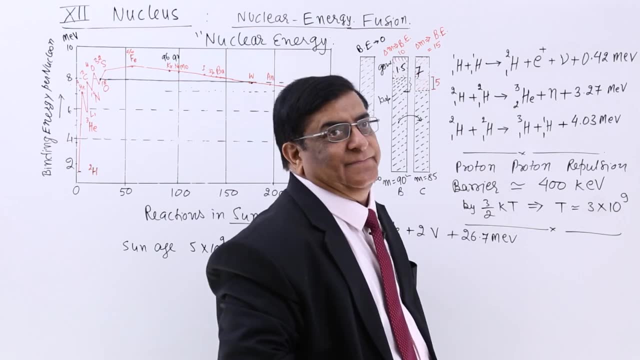 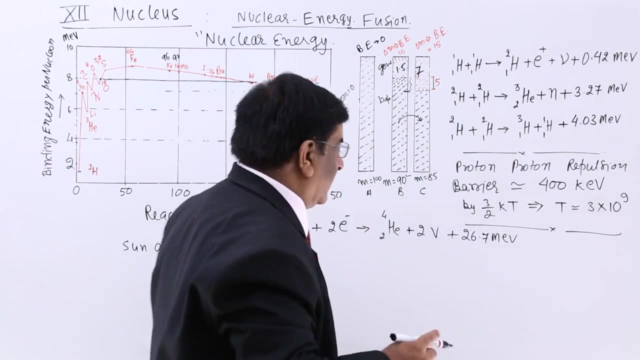 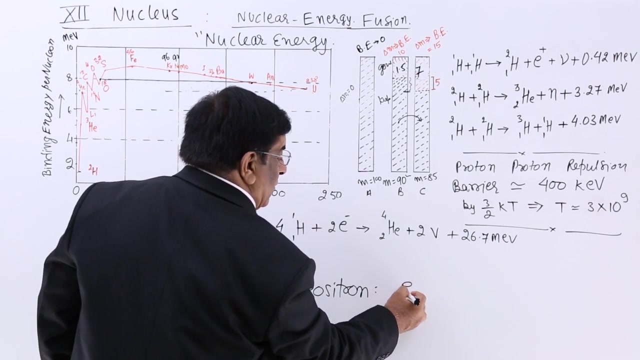 is released, positron is released and one neutrino is released, and there is lot of energy released here. okay, positron, I think we have gone through it. if not, then please do not forget to subscribe to our channel. Please note what is positron: just like electron which has got negative charge, there is a particle. 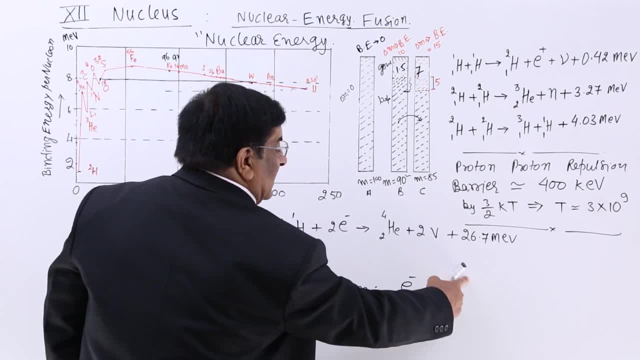 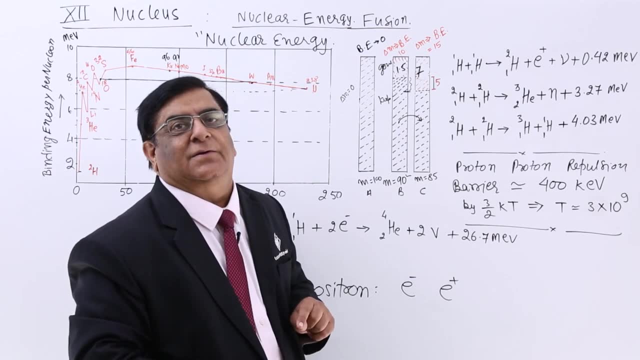 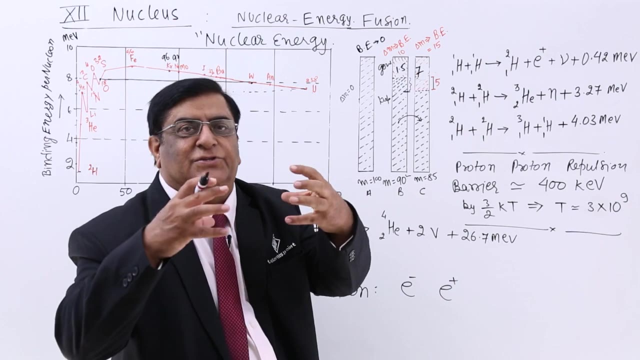 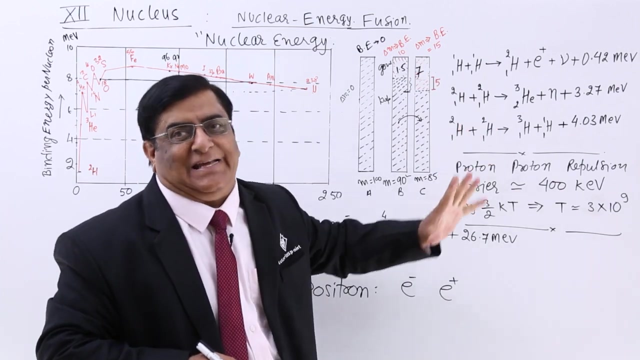 of the same mass but the charge is plus and this is known as positron. this we have studied when we are doing chapter number 1, electric charge. there we had this electron and positron, both the things which they amputate, They embezzle each other and we get energy. that energy we are now studying here in detail. 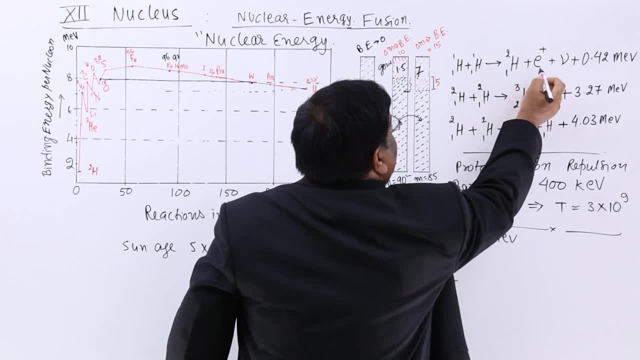 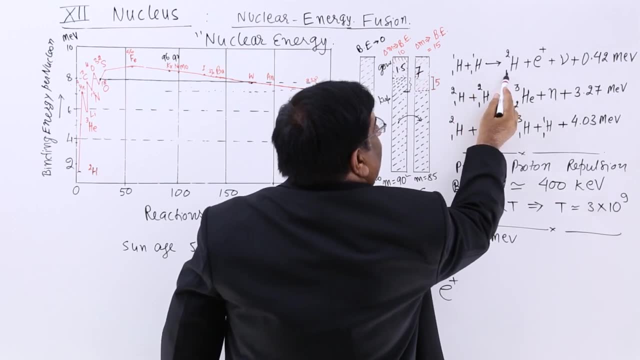 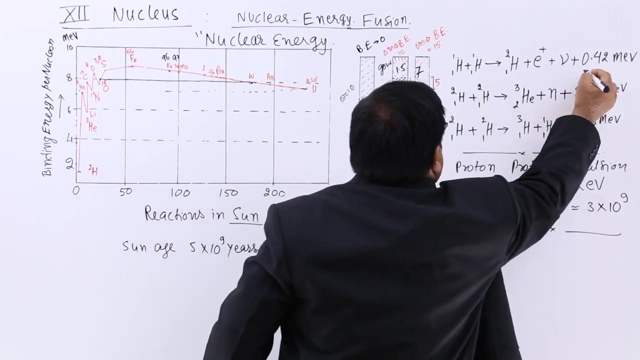 So see, hydrogen hydrogen, they give one positron, E plus is separated and we get this hydrogen. this nucleus has got one positive charge and two masses together and in this process, this process, we get lot of energy, because this was having zero energy, no energy. and in this, 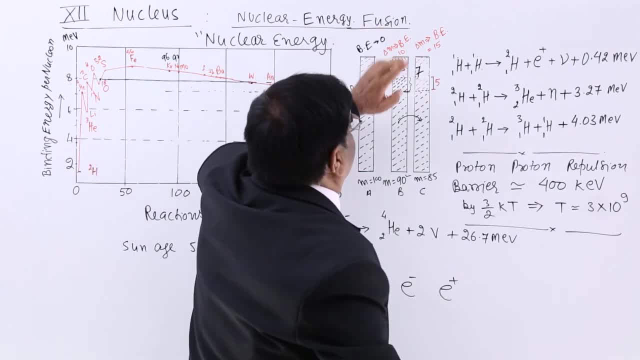 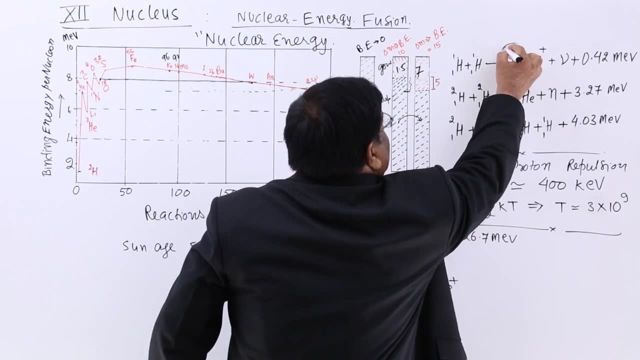 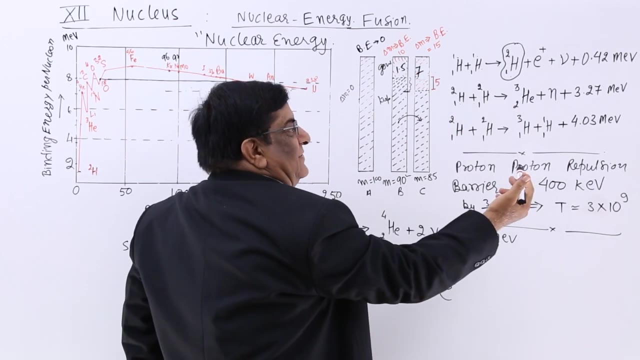 case, then it has got this much정이 wi- Staff of one zurück are reaching full potentialphoria, So we get energy: 0.4 to million electron volt. Now we are getting this, This finished product, again combined with each other in second stage. in this stage, 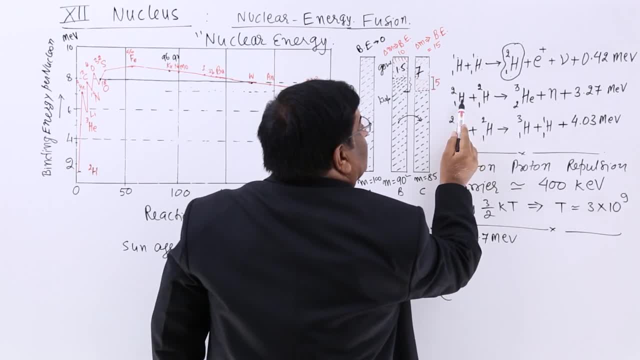 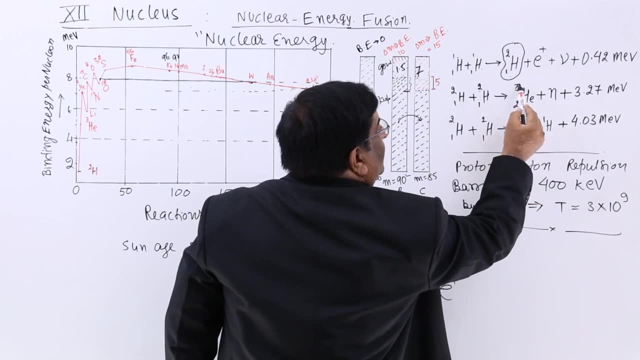 and they combine, then they produce. there total mass is 2 plus 2,4 and we get helium isotope of lose, all the other modulated in the point. Now, what is positron's, Positron's of mass, 3. What happens to that one mass? That is mass of neutron, and it is separated. 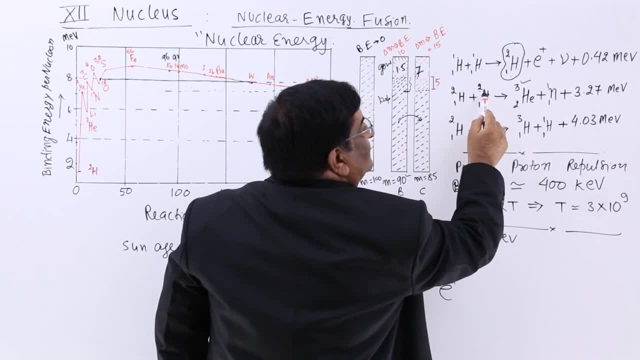 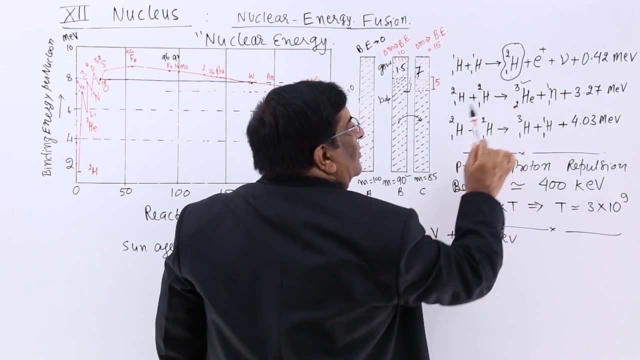 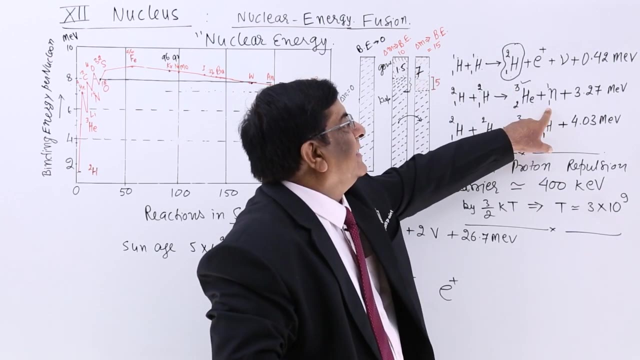 here 1.. So 3 plus 1, 4.. So we get 1 helium, because the charge is 2, its name has changed from hydrogen to helium. The mass: we find 3 and one mass. we find another particle which 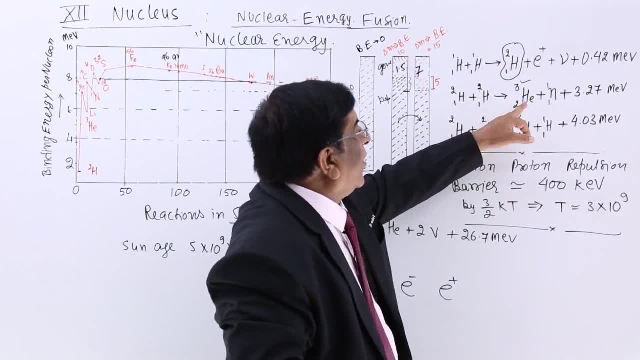 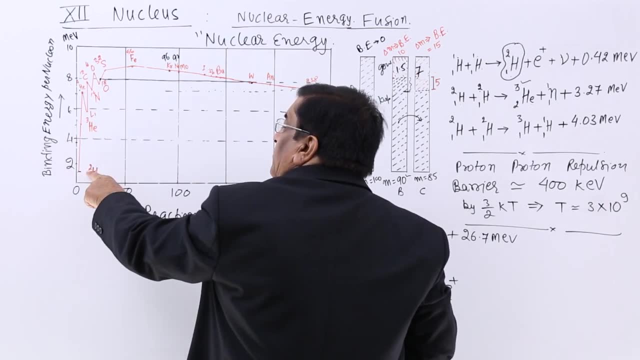 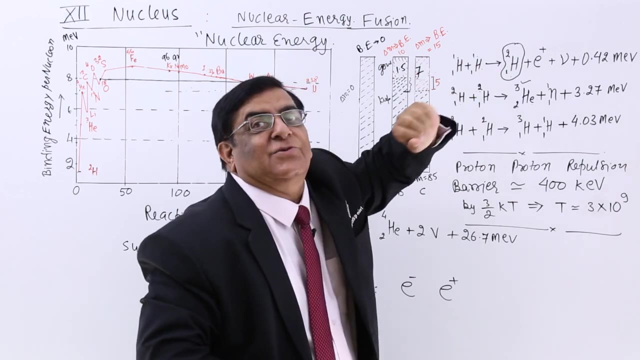 is neutron And in this because helium 3, helium 3 is again higher than 2.. If we go from 2 to 3, we are going to higher binding energy, and higher binding energy means energy is radiated out, released out from the material. So how? 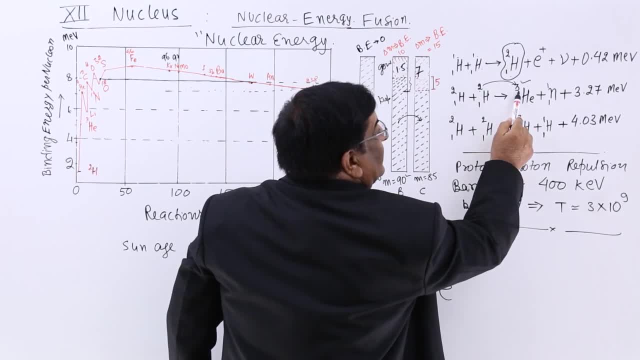 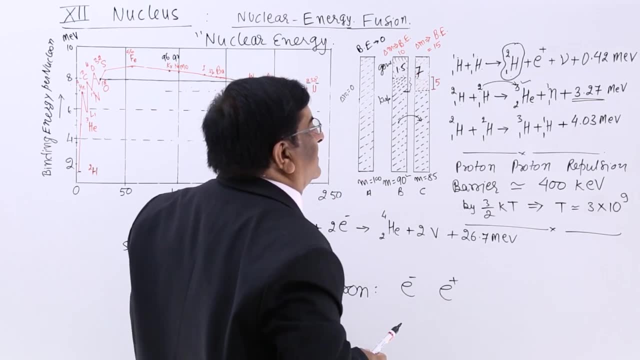 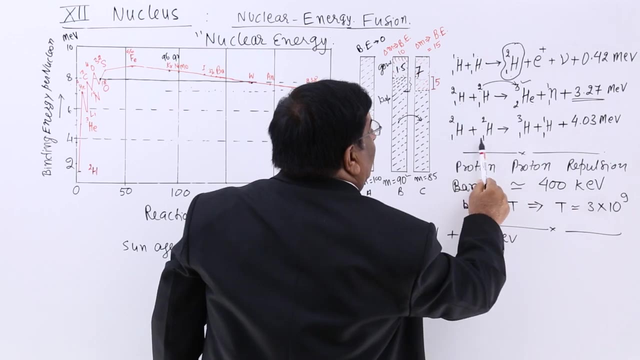 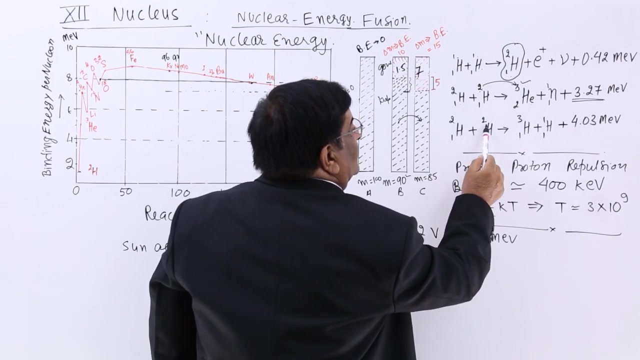 much energy is released due to this. 2 to 3, this is the energy released. There is energy released. So from this we another action: we can presume that if they do not combine to make 2, maybe they remain 1, but this become 3.. So hydrogen 2, hydrogen 2 make hydrogen 3.. Again, there is a change. 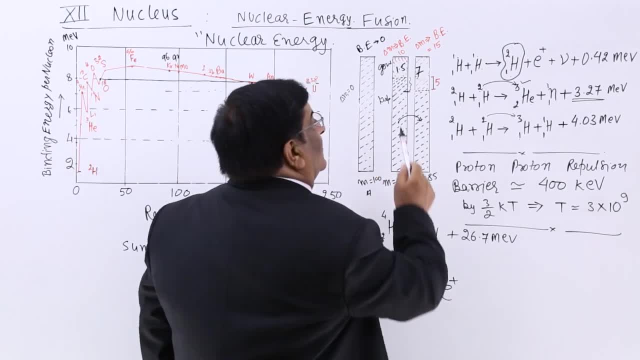 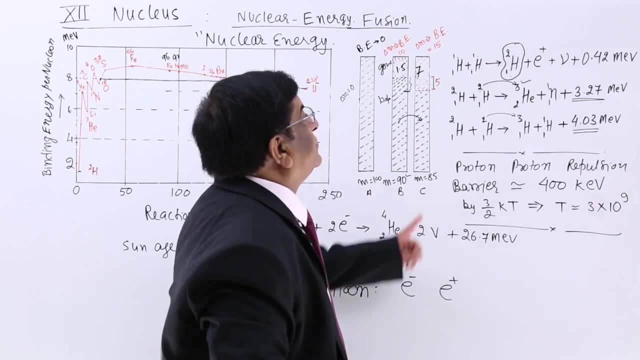 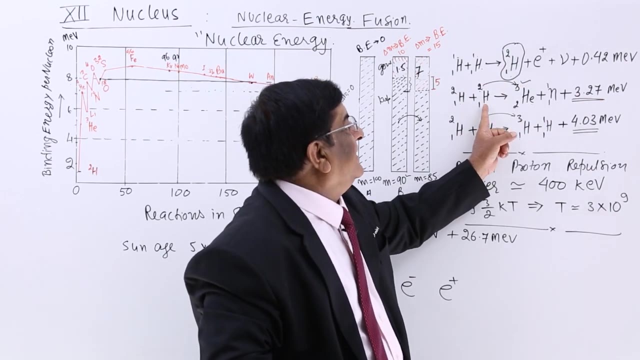 from 2 to 3,, 2 to 3, and there is a gain of energy. This gain of energy is how much? 4 .03 million electron volt. So first this thing happens in hydrogen and what we get here it combine either in this method or by this method. In both the methods we are getting. 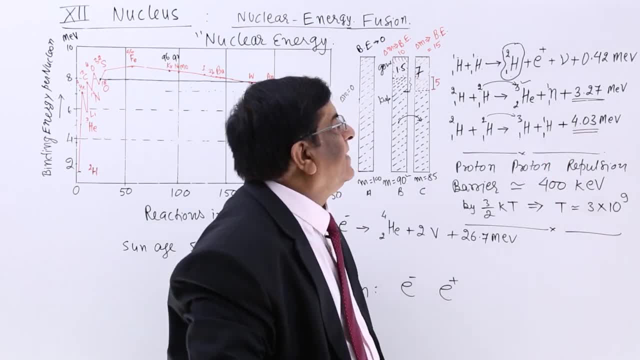 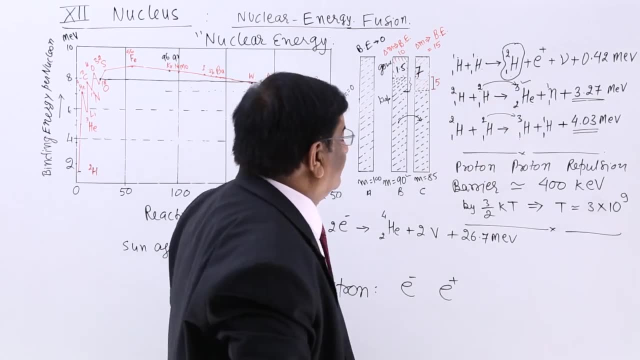 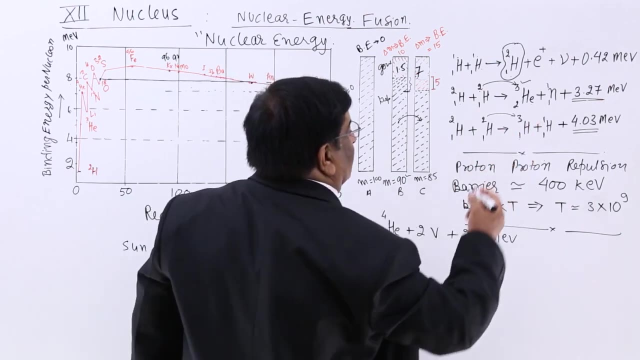 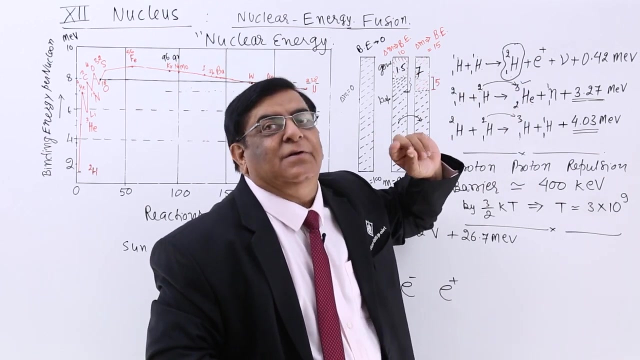 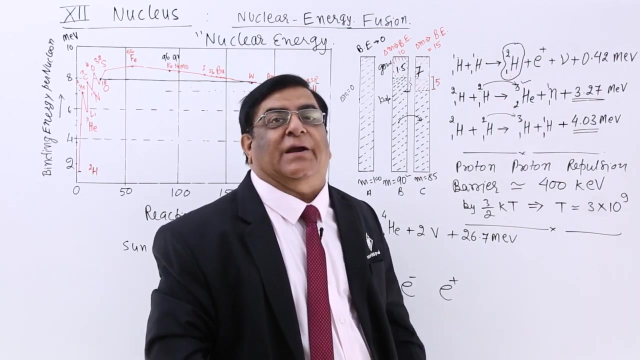 lot of energy. here it is. So this is how hydrogen is converted into helium. Now this is one example of hydrogen. Now, when we expect that we this thing happens by writing equation, it seems to be very easy, but when practically we do it, we find it is very difficult. Why? This is one proton. this 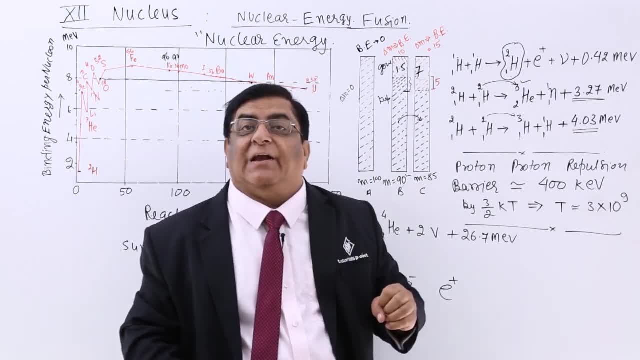 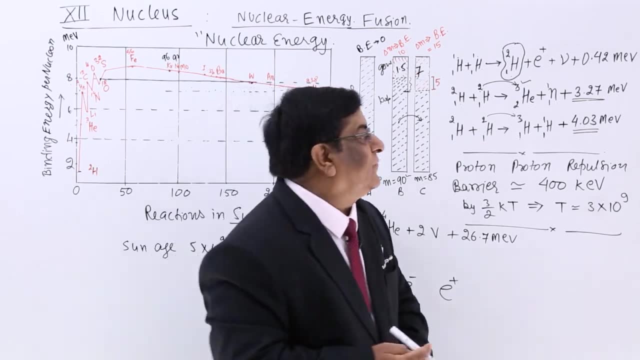 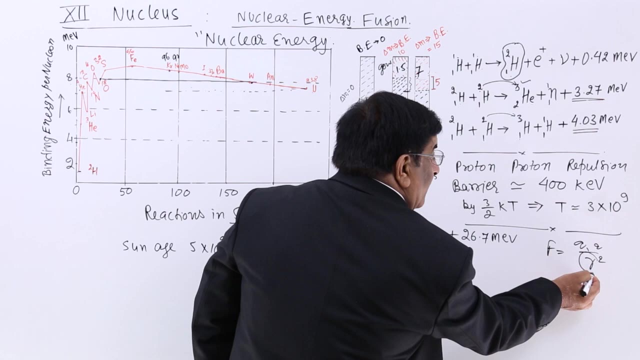 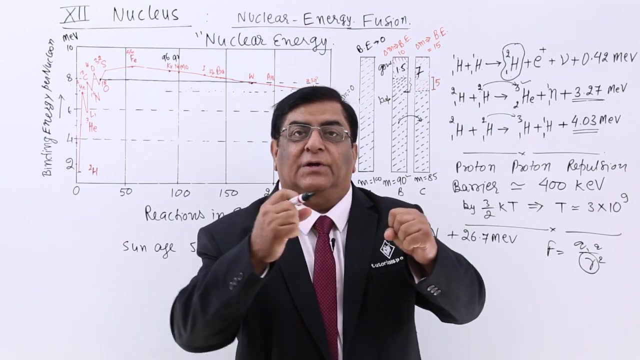 is one proton and they have got positive charge and we want them to come together and fuse. That is very difficult because coulombs force is q 1, q 2 upon r square. This r has to be very, very small, So the force will be very large. To counter that force, their speed should be. 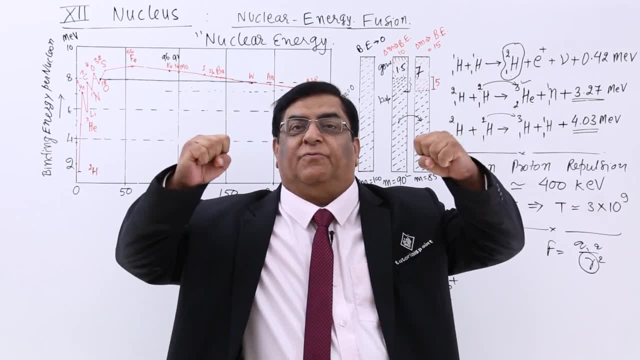 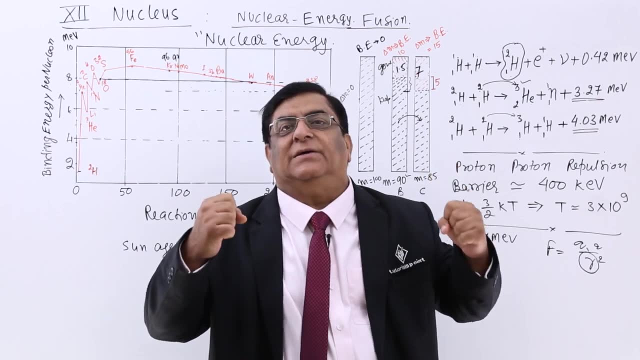 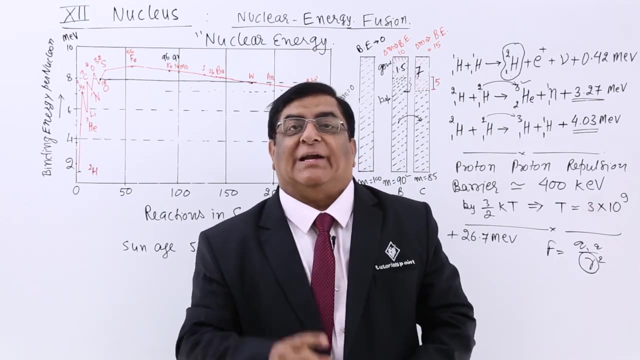 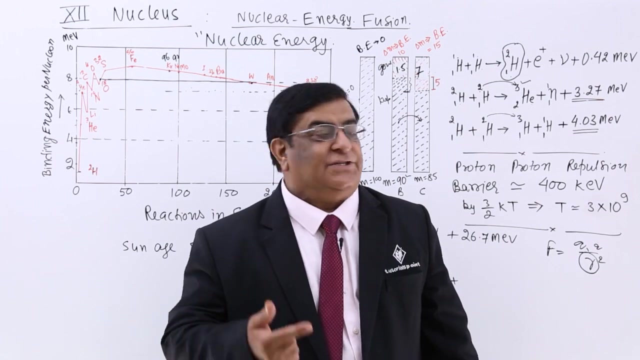 very large, This proton, this proton. they should be very large speed So that before they are reflected by the coulomb force Force, before they are reflected they must stick together. That much energy we should get that, and how much will be that energy? We have calculated it that that energy should. 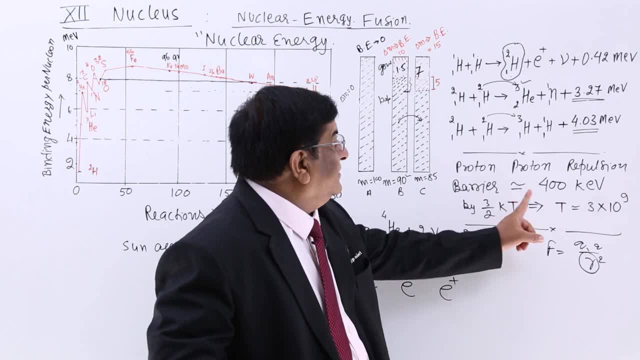 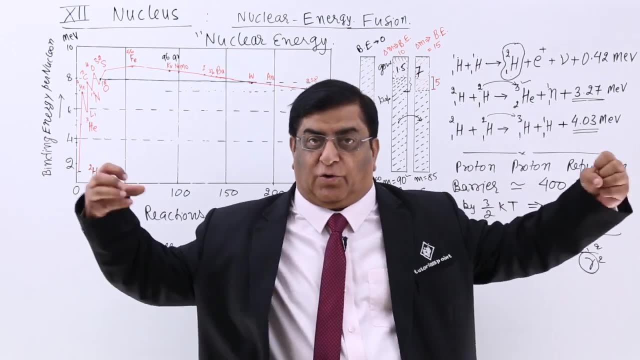 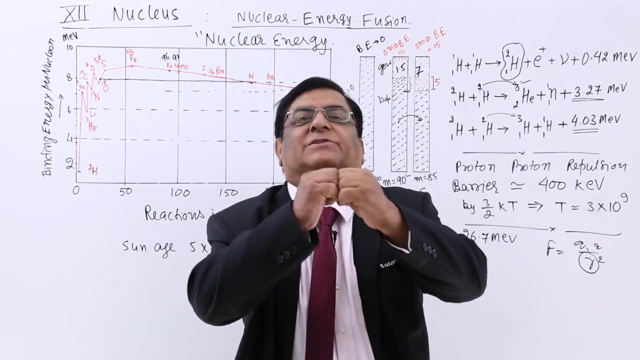 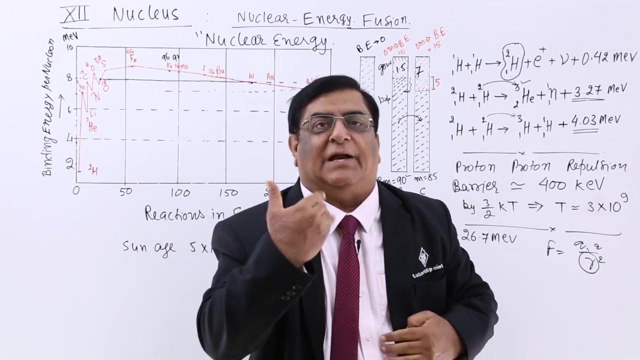 be more than that. energy should be more than 400 kilo electron volt. If we give so much energy to proton, then it will move with so much kinetic energy that before they are repelled They strike each other. They will hit each other and get fused. Now how to give that? 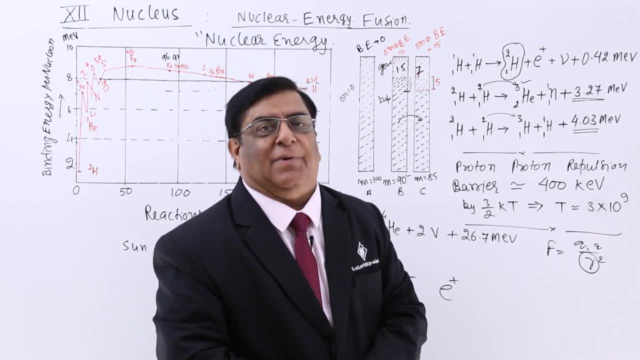 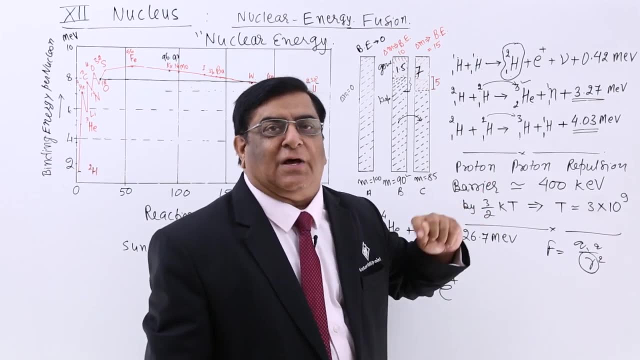 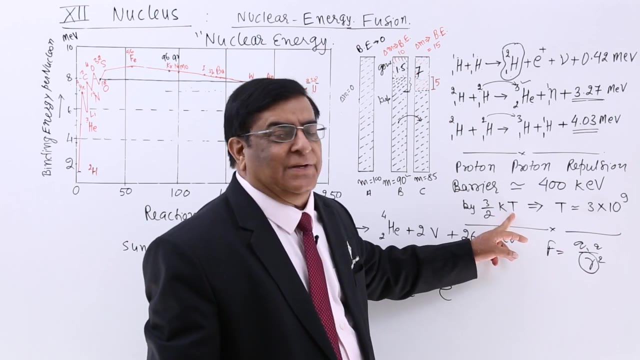 much energy? The answer is that energy is given by thermal energy, by raising its temperature. How much should be the temperature? So for thermal energy we have a formula 3 by 2 k T. You all know this formula, It was in the gas equation. So by this, if we put this energy, 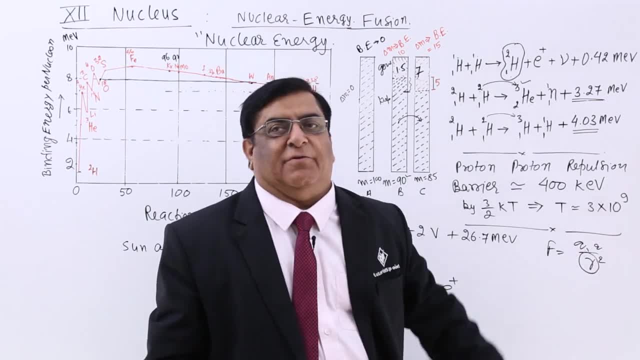 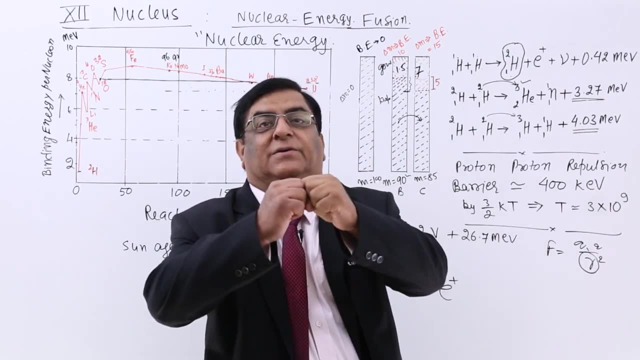 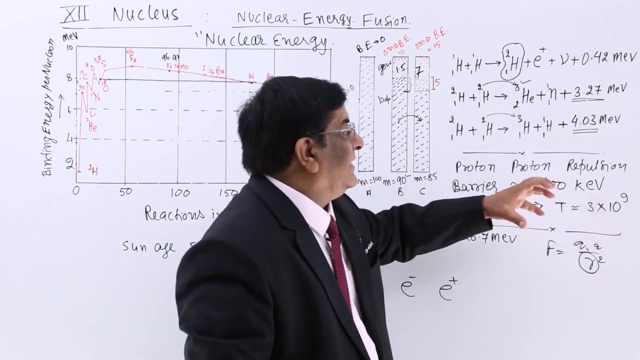 we get the temperature to the order of 3, into 10, to the power 9.. So we need that much high temperature if we want to fuse hydrogen converted to helium. This is the way we have to, that much high temperature is required and that high temperature is not possible. 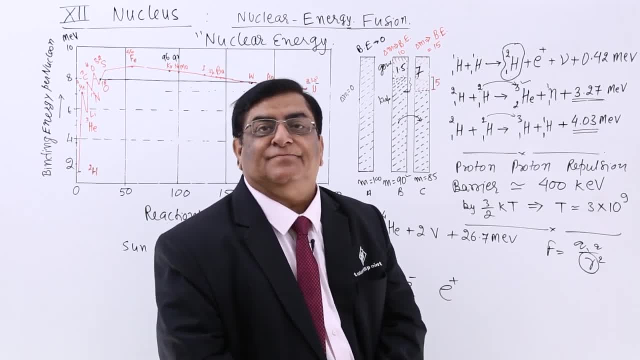 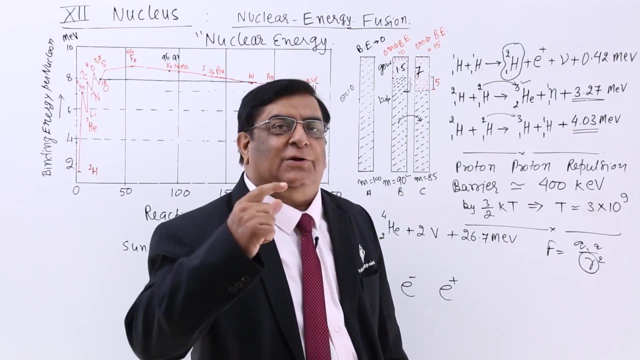 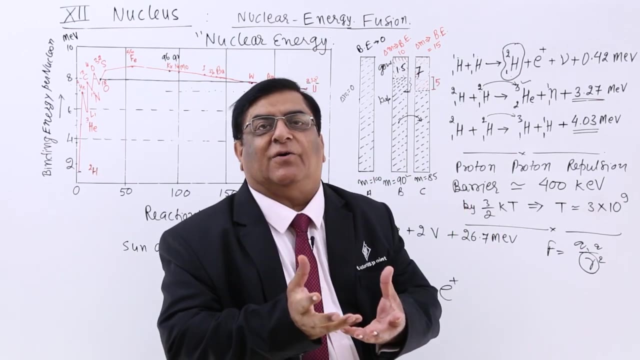 for anything on our earth. Then what do we do? Okay, We have studied this. We have studied one process before this. That was fission process. So we start a fission process in this chamber of hydrogen, Hydrogen, hydrogen. it is kept in a chamber and inside we have 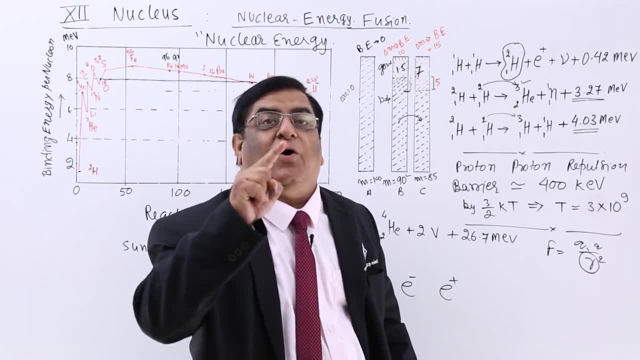 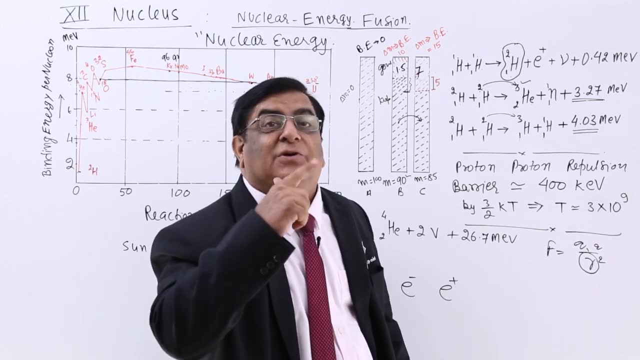 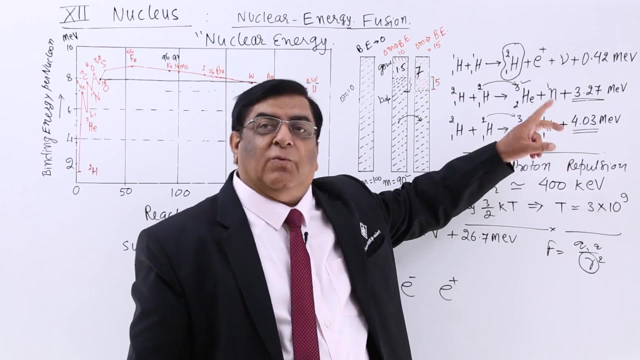 a nuclear bomb. What is that Fission process of uranium? That fission process is having so much energy that temperature rise to cross to 10 to the power 8.. More than 10 to the power 8.. This much temperature is achieved When this temperature is achieved. then hydrogen start combining and the moment they combine, lot of energy is released and this energy is very, very high, much higher than the fission energy. Now, when this starts, then it starts burning itself. Now it does not need fission to raise the temperature. Who is rising the temperature now? Hydrogen itself, because so much energy. 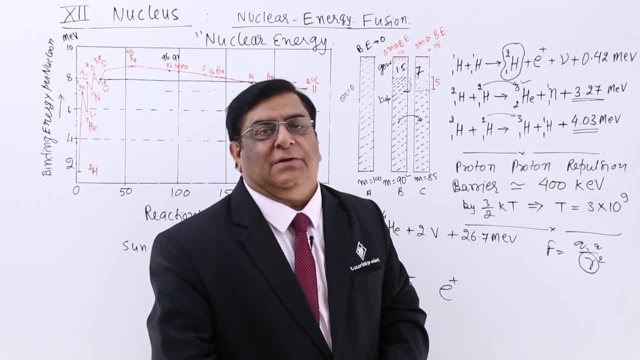 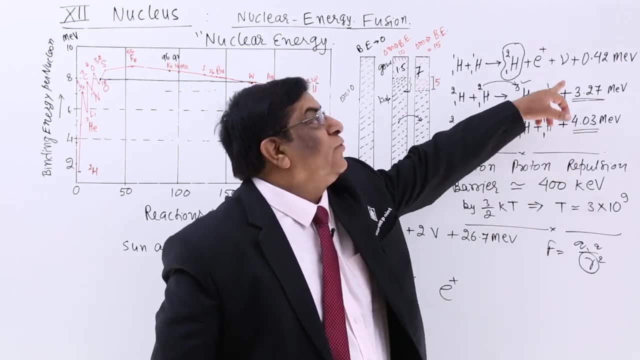 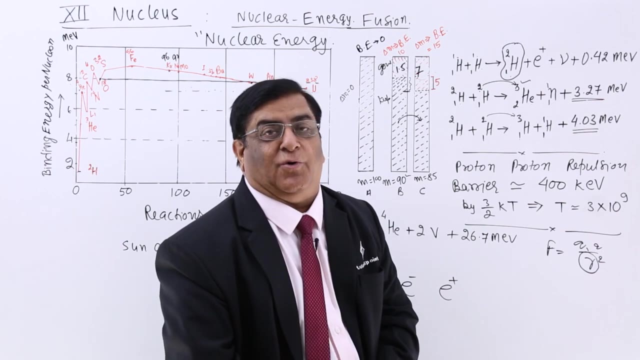 has come out and then we cannot stop it. Whatever is the complete hydrogen has to burn, has to fuse and will have to give so much energy, heat, So much heat has to be there. So if you make a hydrogen bomb, it is very, very destructive compared to fission energy, because you see, 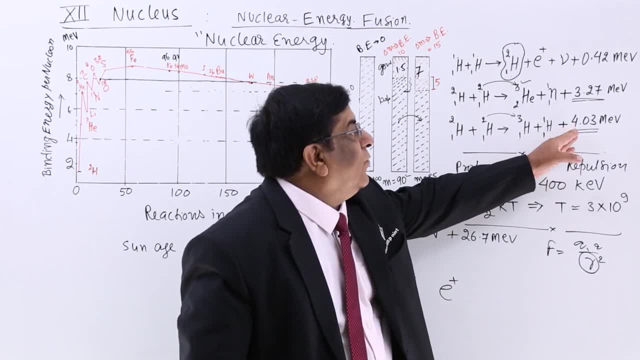 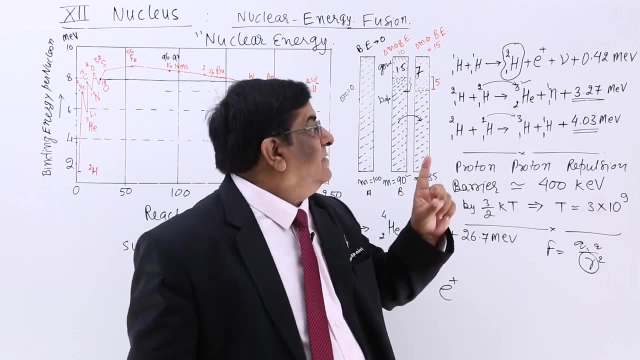 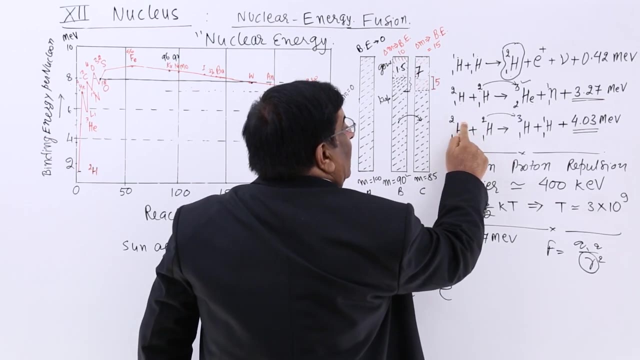 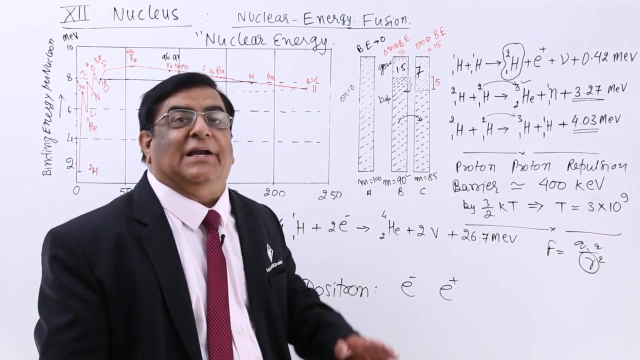 it is giving how much energy. This is giving us 4 million electron volt for one, and for this we can say 4 for 2 and 2.. This is mass, atomic mass 4, and we are getting energy- 4 million electron volt. and when you go for fission process, the energy is much less. you have seen. 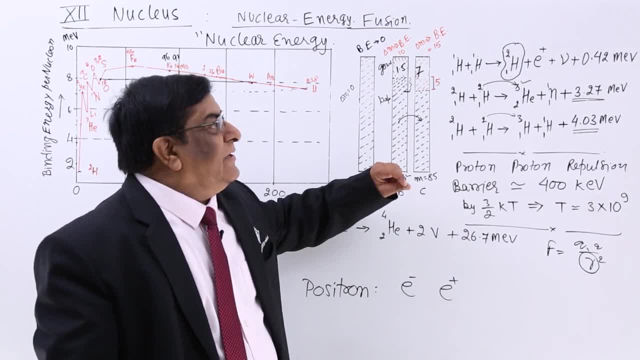 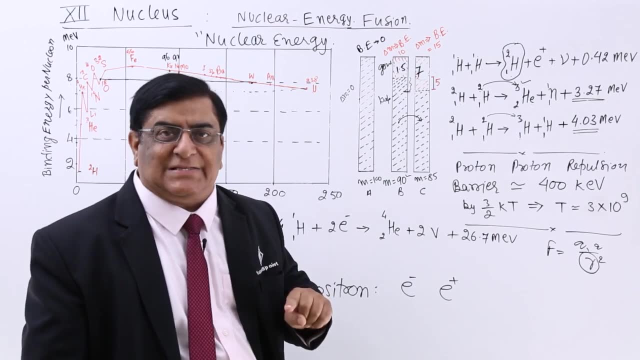 in the previous lecture. So we have finished. So this is the final technique, So we will continue further. Thank you to the fission. if we go for one nucleon energy in, fission was less one nucleon energy in. hydrogen combination is larger. So which process gives more energy? Answer: hydrogen fusion gives the more energy. So that is why hydrogen bomb gives more energy. So this is about the hydrogen combination. The source of energy for our nature is sun. 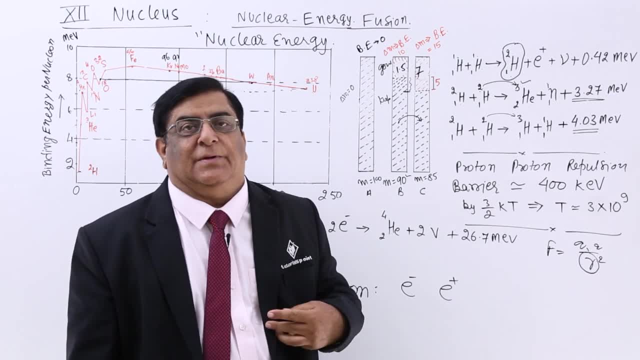 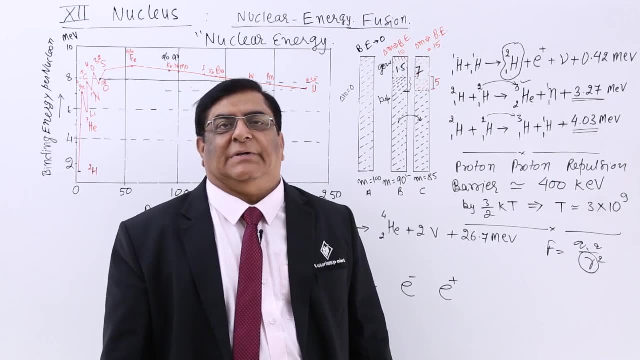 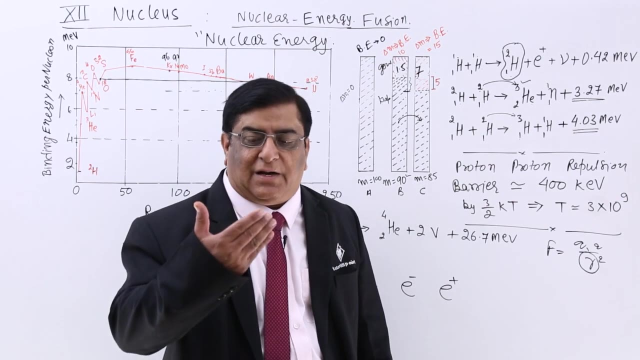 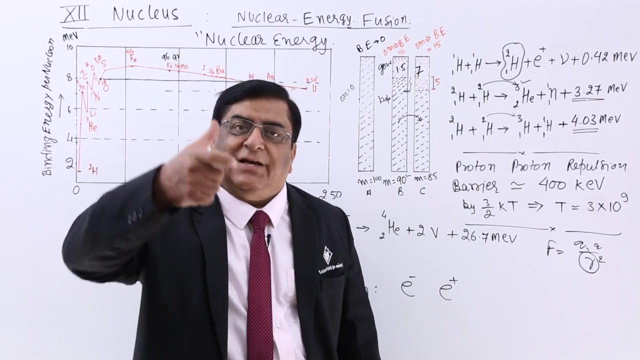 In the sun how energy is produced. We think we analyze that sun is full of hydrogen and helium. So we think the same process is happening in the hydrogen and there are proof. there are proof in the light of the hydrogen burning, That is, in the sun, in the spectrum, the light. 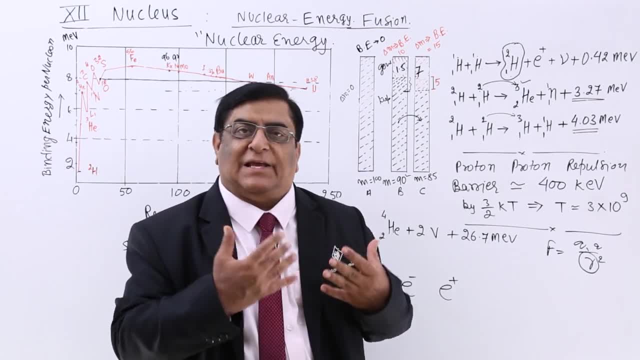 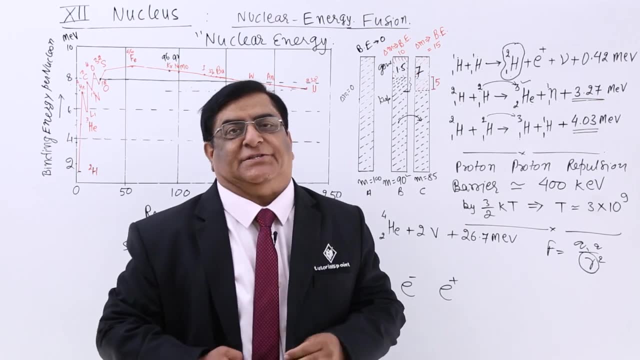 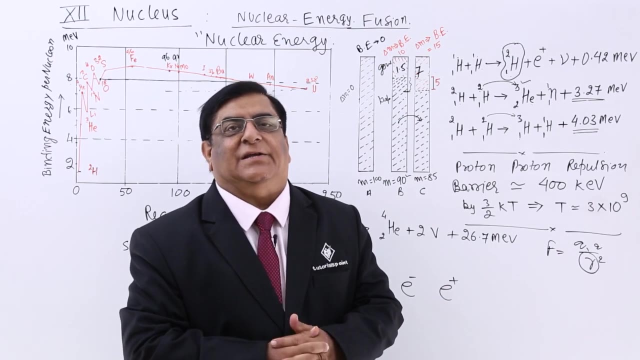 coming from the sun. when we analyze here, it is the same type of a spectrum when we get hydrogen burning on the earth for different temperatures And that gives us outstanding evidence of this heat idea, of the temperature of the sun. and that color of the light gives us the idea that 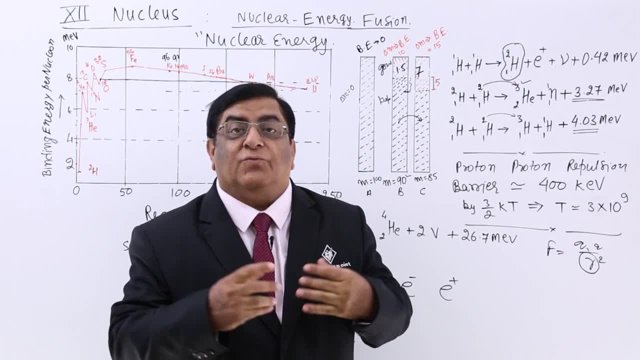 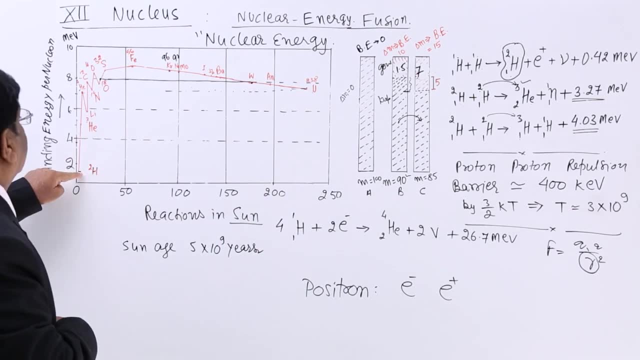 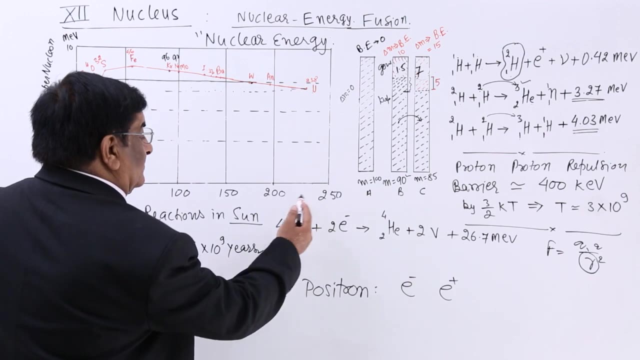 it is hydrogen which is burning in the sun. So we think that hydrogen there which is converting to helium. hydrogen converting to helium gives us energy and we get the equation this way. There are again different categories, but finally, when we sum up what we find, that 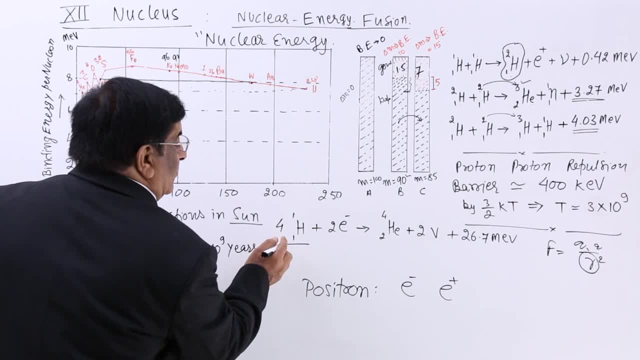 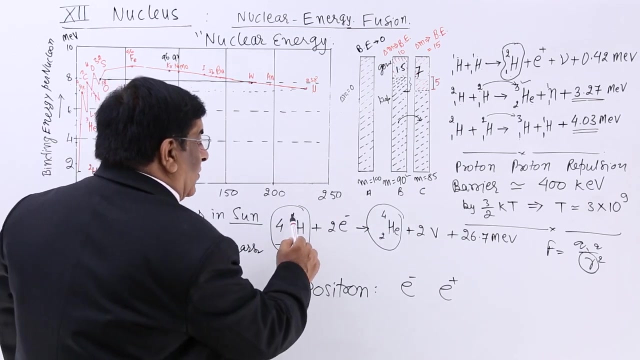 4 hydrogen nucleus: 1: 1 make 1 helium nucleus, 4 hydrogen. 4 ones are 4. this is 4.. So 4 mass of hydrogen makes 1 helium. Other things So there are 4, quelitos are additional, it does not matter. So hydrogen to helium, that. 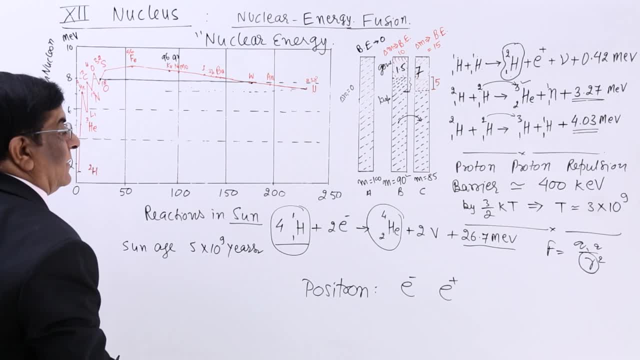 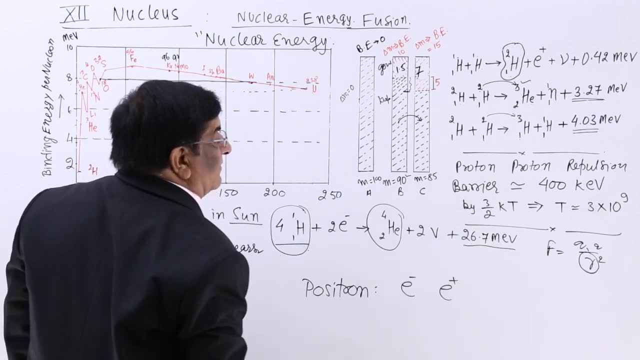 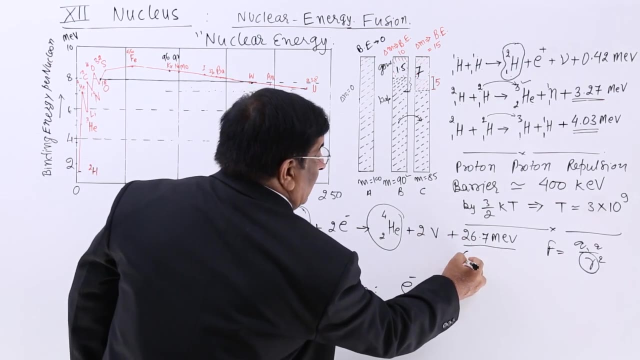 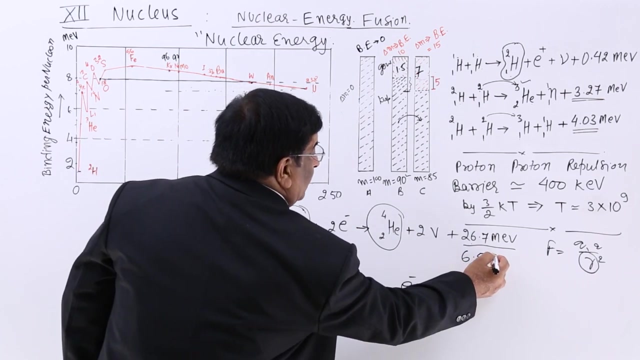 gives us lot of energy. this one, And how much is this same 4 Particle of hydrogen has given us 26.7 million electron volts. So what is 1 hydrogen giving? 1 hydrogen, nearly nearly 6.5 M sneaking of hydrogen. 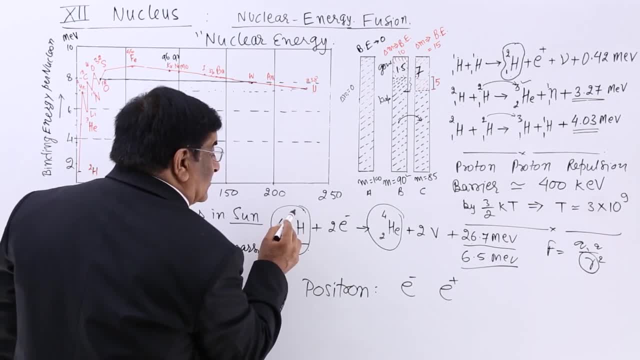 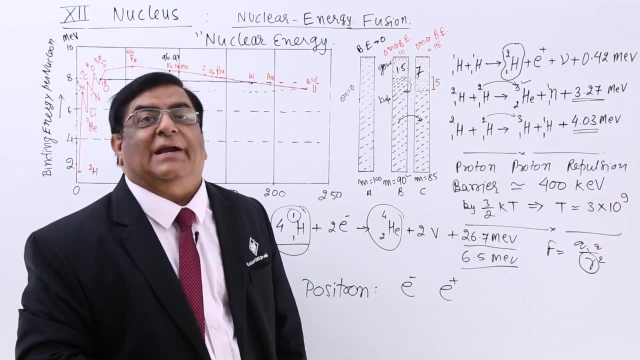 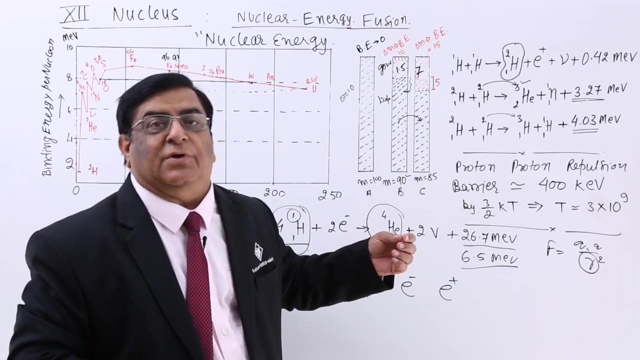 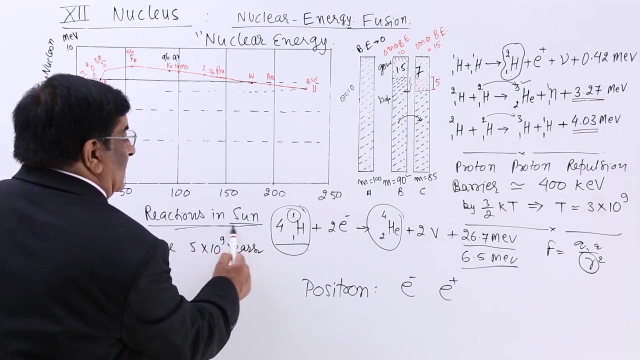 electron volt for 1 hydrogen, 1 nucleon of hydrogen. it gives so much of energy and in the fission we write it is 0.9.. So this is a much more effective and much more economical means. it gives much more energy. ok, So this is the reaction in the sun. please remember. 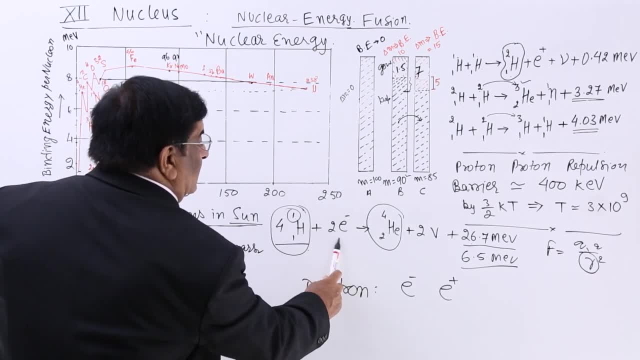 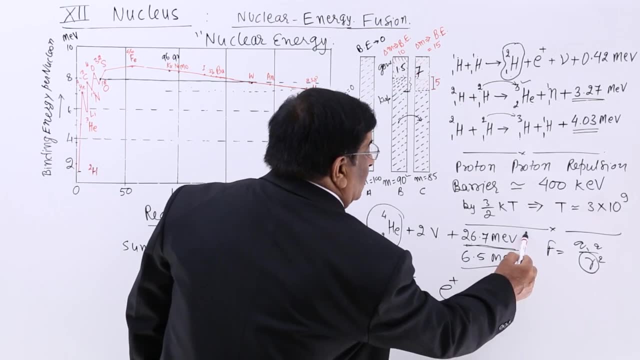 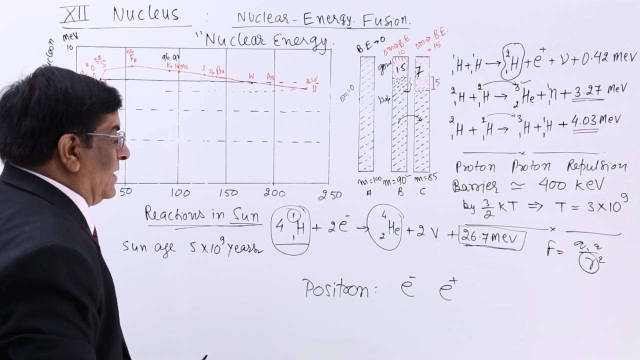 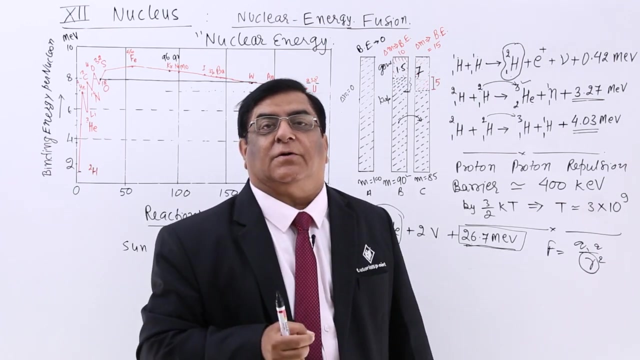 this reaction, hydrogen mixed with electrons, make helium 2 neutrino and such large amount of energy. this is source of energy in the sun. ok, So there is a huge stock of hydrogen and helium in the sun and this will last for another 5 seconds, ok. Also, this is the reaction in the hot gas period. it rises throughout. 5 billion years. The sun still has not crossed this half life and still there is lot of life with the sun. it is quite young even at present. So this is fusion process which is happening in the sun. basically, we have seen this type of processes here and the same process we 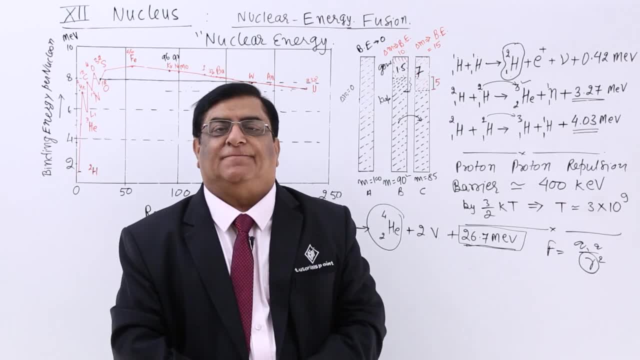 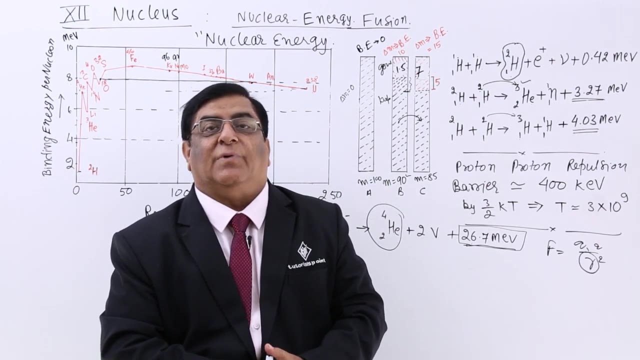 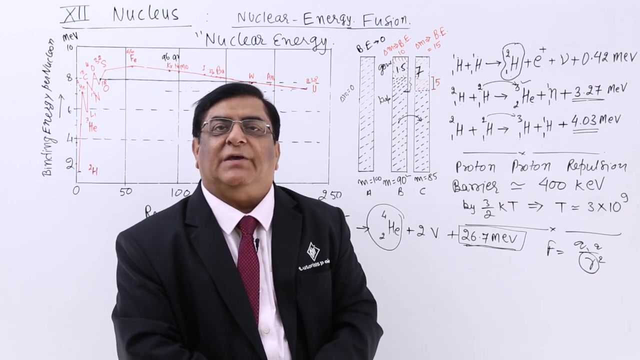 can do under controlled conditions on the earth. When we do it under controlled condition- hydrogen fusion- then we call it hydrogen bomb and that is so. many trials are being done on that to get energy from hydrogen by this way, because this is the maximum energy we can harvest, But so far we have not been succeeded to get this energy for our useful purpose. 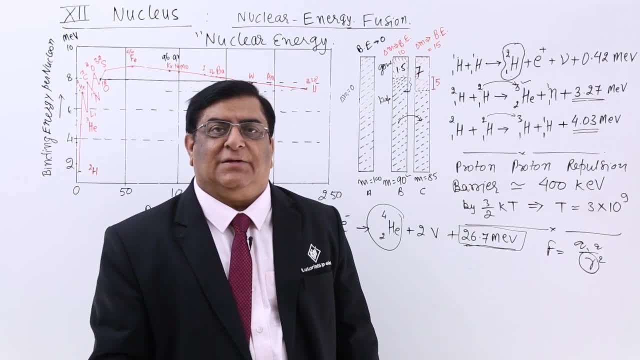 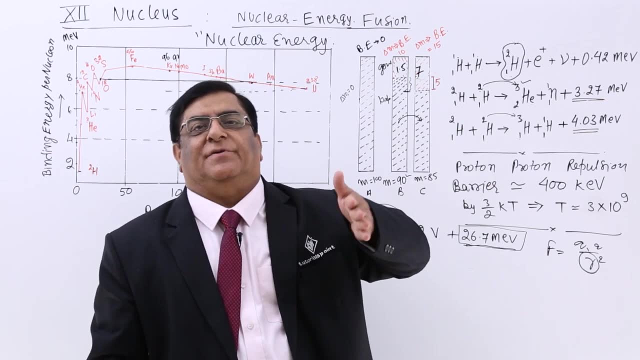 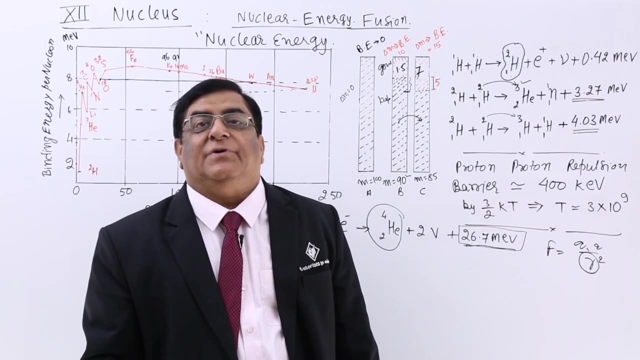 For the fission. we have made fission reactors. the energy output from fission reactors we are using to make electrical power and that power we are getting from the reactors. But fusion so far we could not make any reactor. we have not developed that technology. we know. 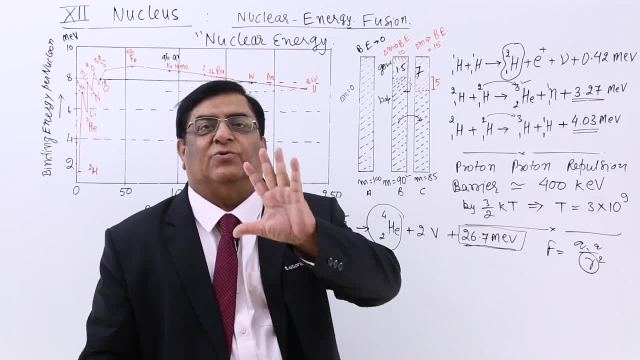 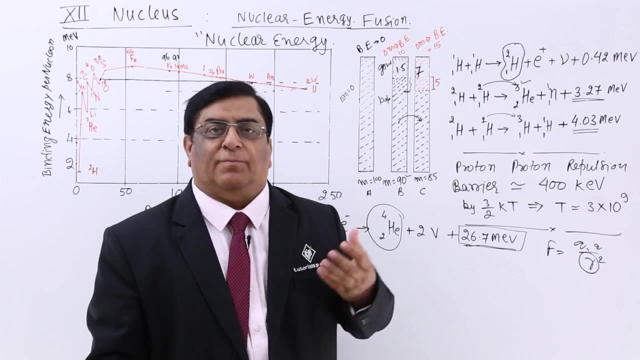 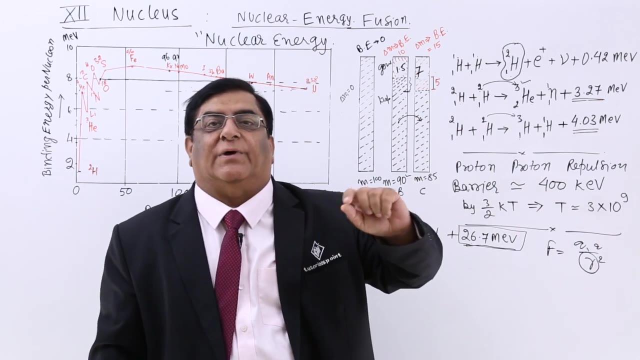 the principle. we know the reactions, but technology we could not develop So that we convert this into useful energy. So may be in future. we are trying for it. there are reactors in which hydrogen fusion will be used to get the energy. Why should we favour fusion energy compared to fission? 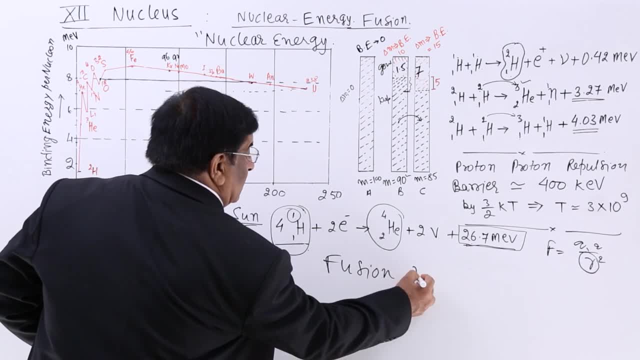 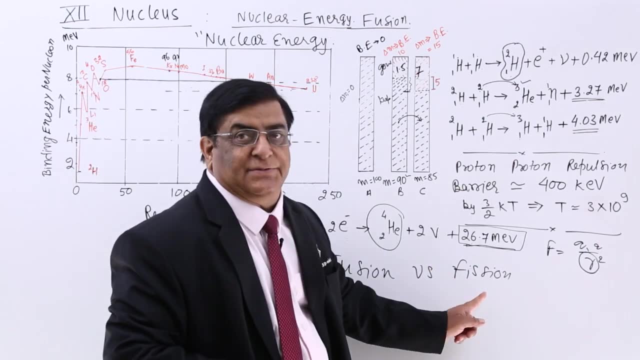 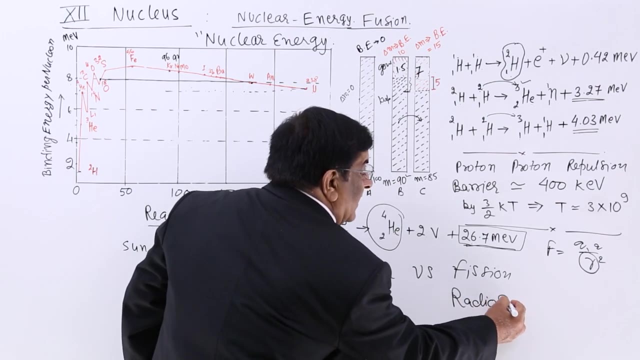 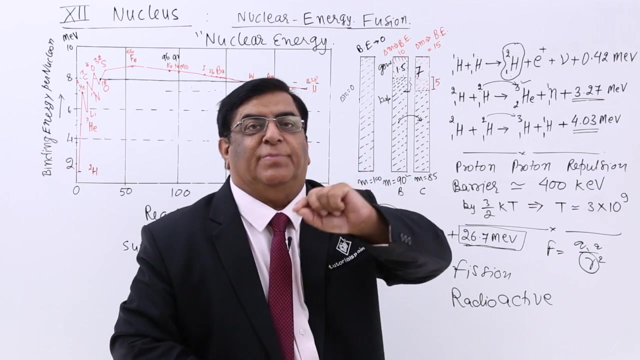 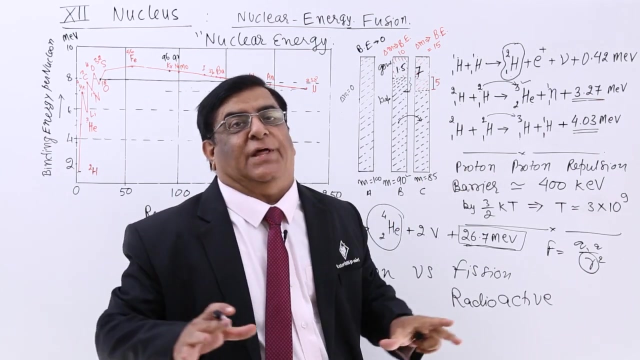 energy Fusion versus fission. in fission there are many problems because this is due to radioactivity And products we are getting are still radioactive And those products, when they are giving out beta particles and gamma rays, then this is damaging everybody around them, The atmosphere. 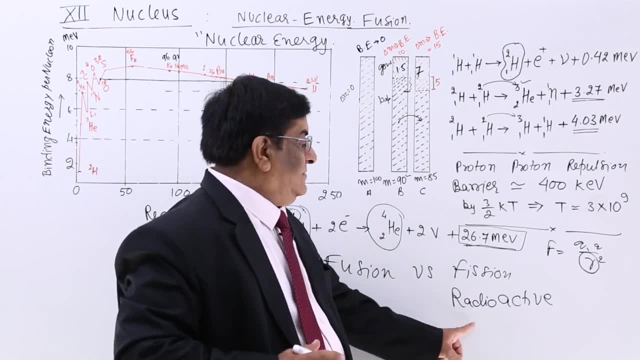 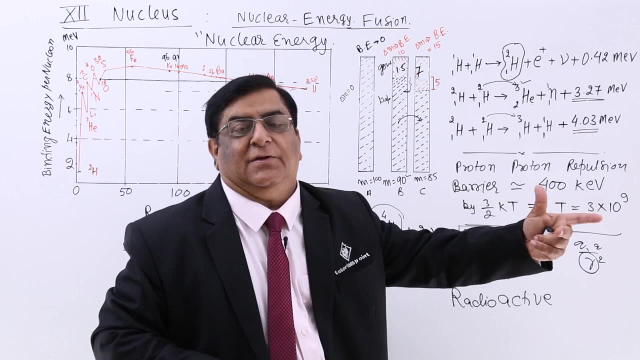 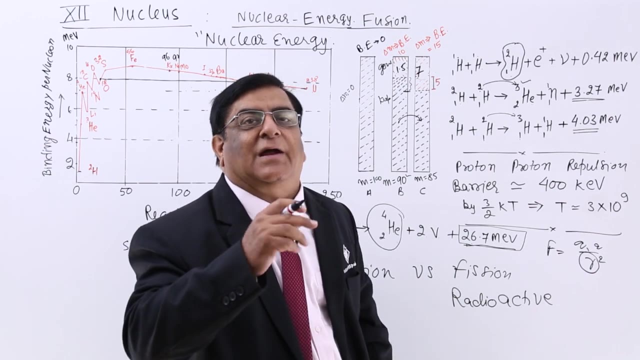 the people and the whole generation is damaged by this radioactivity of the fission reaction And all the products of the fission reaction, whether it is Krypton, SB, NB, whatever it is, that is further radioactive and they are emitting beta particles and gamma rays which 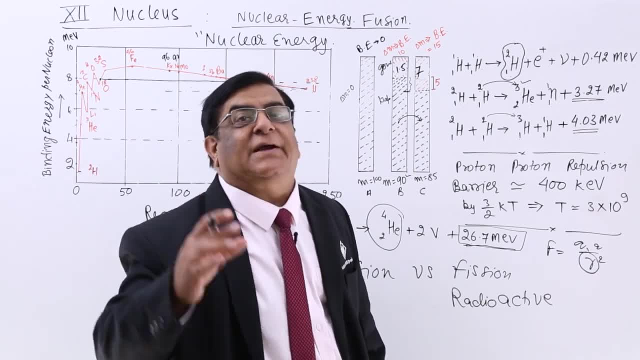 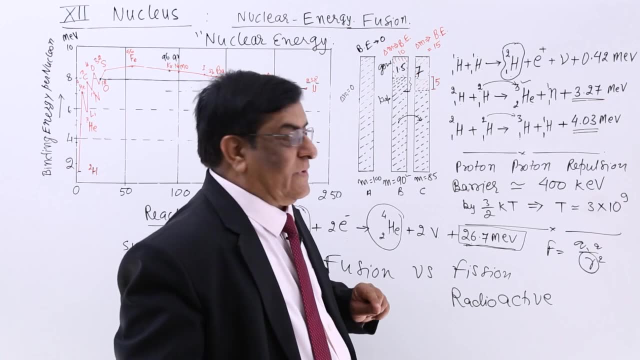 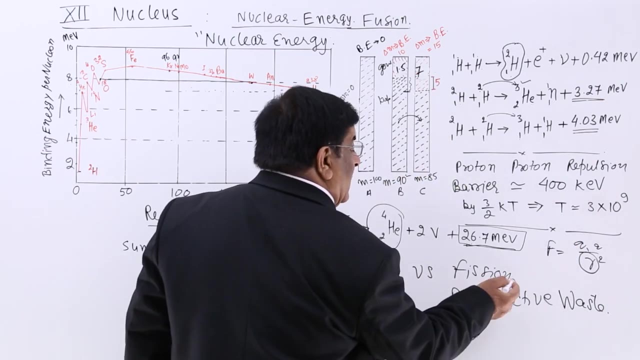 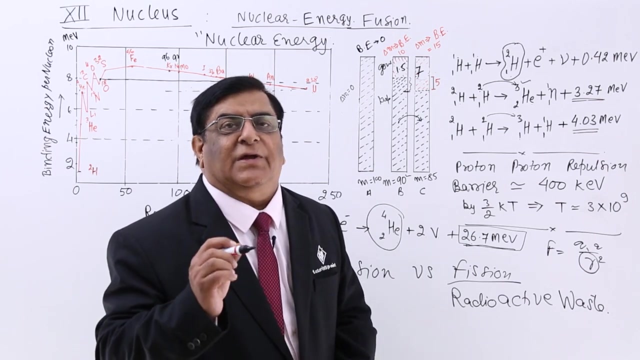 is affecting for years together, affecting everything around it. So that is the danger of fission. okay, So that radioactive waste is our main problem. Other problem is that we want to do fission with U-235, and U-235 is very small in quantity. 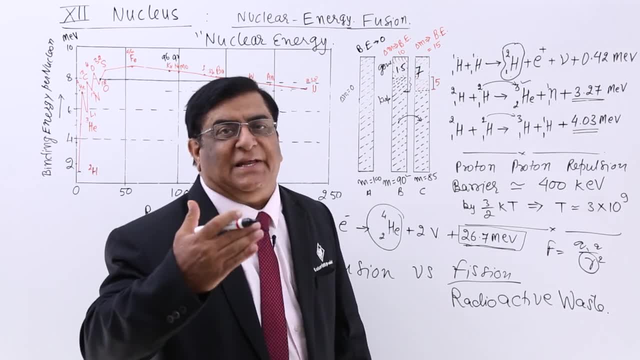 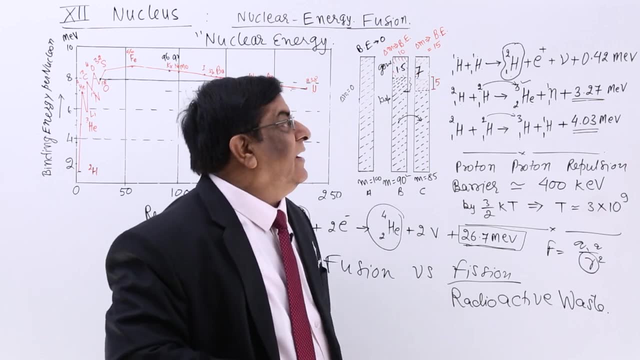 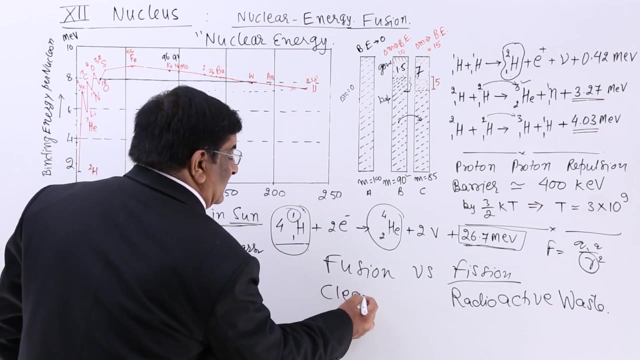 present on the earth. So this is also depleting and after few years may be 100 years, more than 100 years, but it is also going to deplete while hydrogen is in plenty. The benefit of fission is that this is clean. There is no radiation in the atmosphere. there is no radiation. 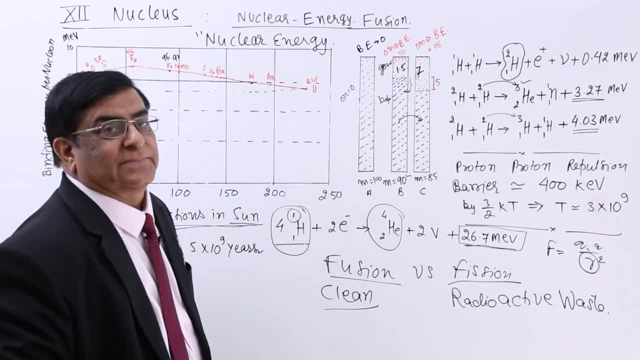 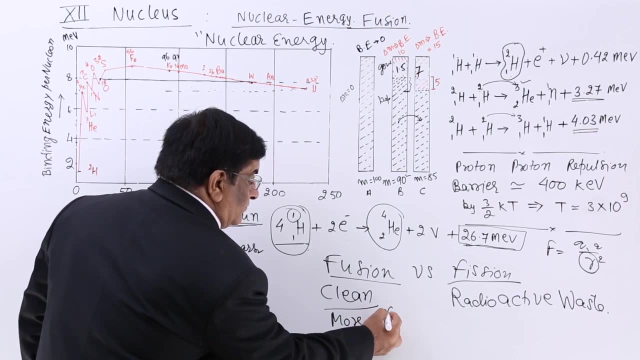 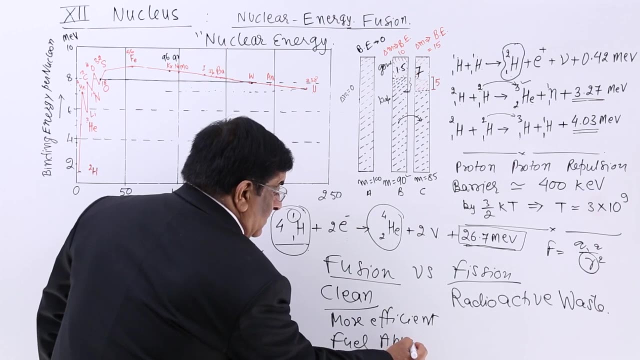 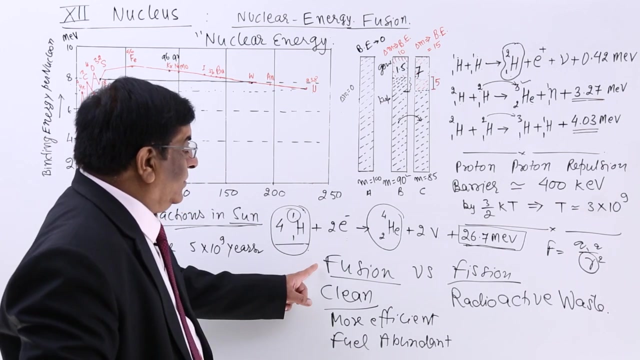 or radioactive waste in the fission process, and that is the main advantage. Plus, it is more efficient, more efficient, Fuel abundant. We have got a very large stock of hydrogen, So that is why fission energy is much, much, much better than fission energy. 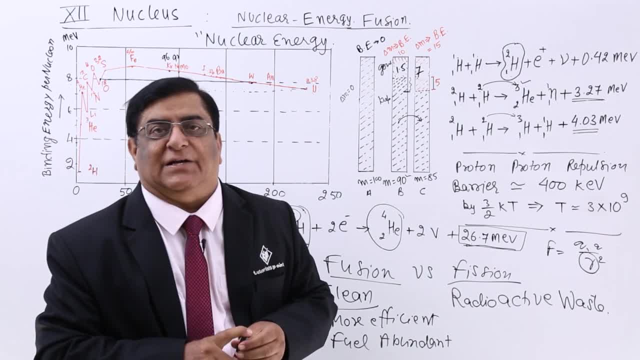 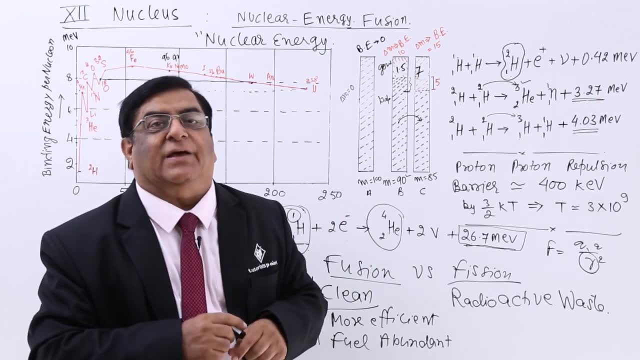 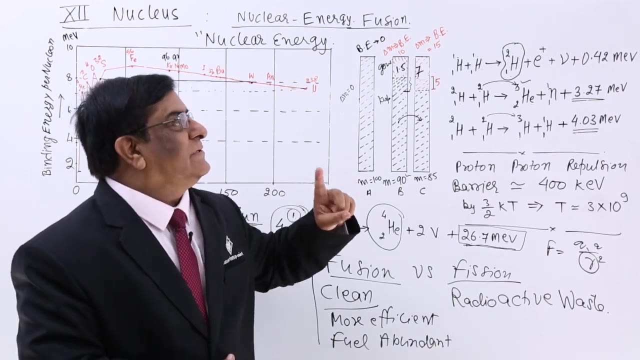 Fission is not seen as a good energy because of its radioactive waste, So we have to make it in a controlled manner. That is why nuclear reactors are kept very, very simple. So this is about nuclear energies, fission, fusion, both the process. Thank you.